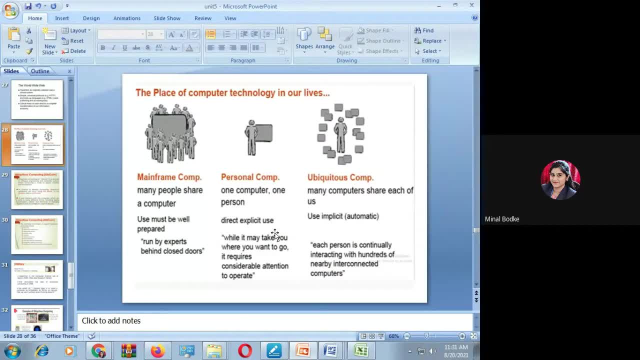 You can have a high-end servers, workstations, laptop. Okay, So in this way the computer get in the. in the second era, the user and the computer interaction was increased. So now, last one, is what your ubiquitous computing? 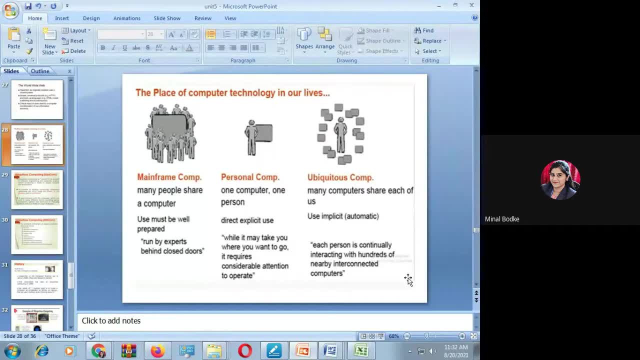 This is the current era We are leaving. Okay, so can you see from the diagram, many computers share each of us. So what is in this? many computers, many users. Okay, so here n number of people and n number of computers can be interconnected. 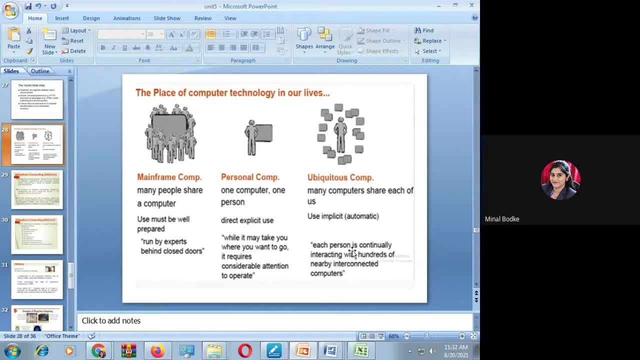 Okay, so that automation of the task can be done. Okay, So this is a concept you have in what ubiquitous computing. So in this, the interaction between your user and the computer has increased tremendously as compared to the basic versions. So in this, the interaction between your user and the computer has increased tremendously as compared to the basic versions of your computers. 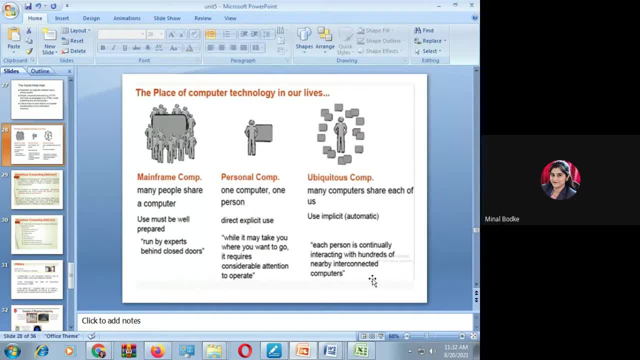 Okay, so what is there in ubiquitous computing? You can take the example. Can you tell me the example? So I can tell you a simple example of you will get this computing is your smart homes. Okay, Nowadays you have a smart homes. 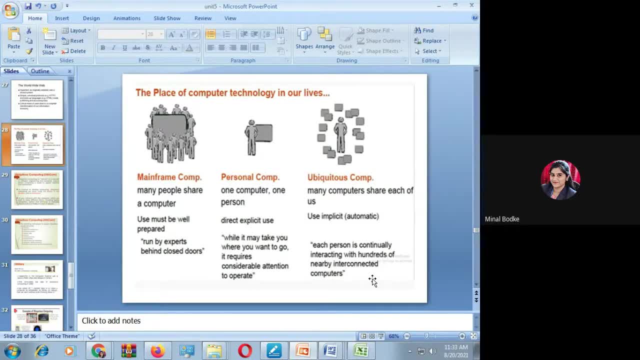 For example, if you move outside of your house and it is too hot, Okay. and again, when you reenter your house, Okay. and if it is a smart home, Okay. and if you have sensor at your homes, using smart homes. 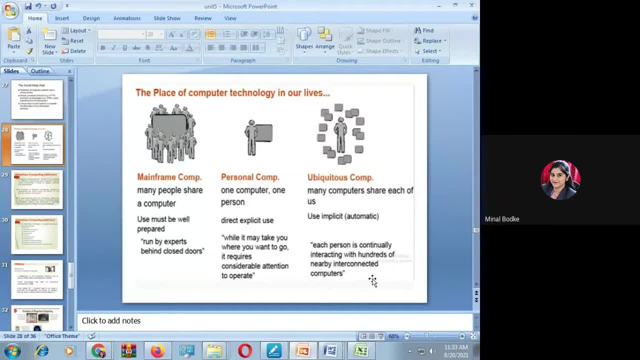 So what the sensor will do? it will detect your body temperature, Okay, and sensor is having some threshold value, So it will detect the temperature of a person who is entering the house and according to that, he will switch on the AC or switch on the fan. 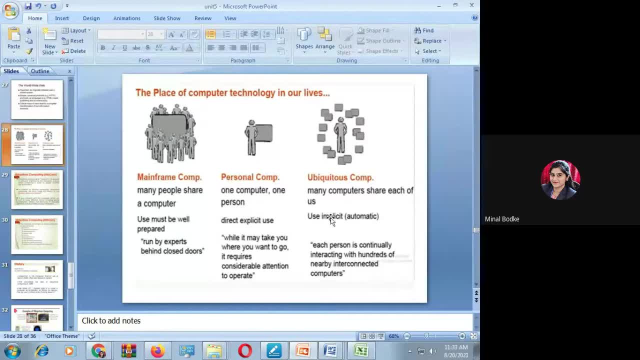 Okay, So how it is done. So in this, can you see, in the ubiquitous computing or in the smart home, There is no need to give any instruction For the human being. Okay, the computation is done whole and sold. by what your computer systems? 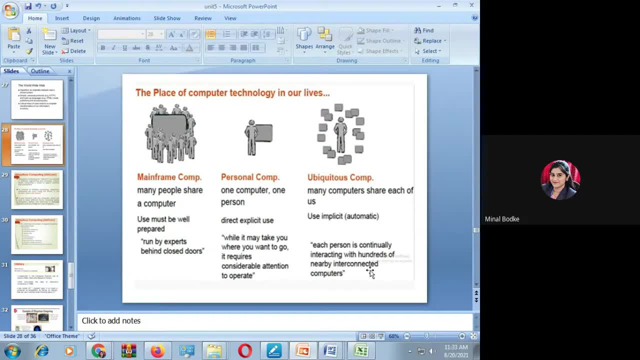 Okay, or the machines or the sensors: Okay. So because of this, what is the advantage? Okay, So the interference of the human has reduced here and automation of the task has increased. Okay, and the user has came more closer to the technology. 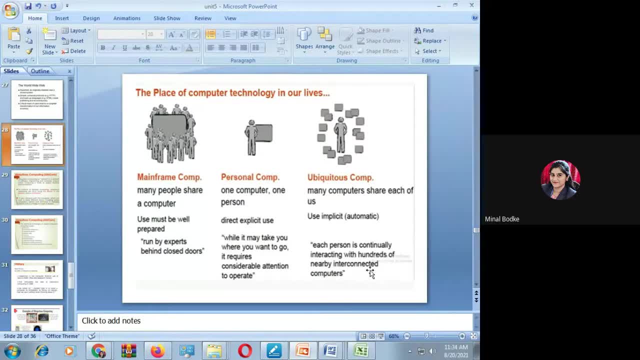 Yes, Can you tell some more example of smart home? Yes, example of smart home. I think so. Everyone is familiar with what is the concept of smart home. Yes, one more example we can say is that light switch on and off. 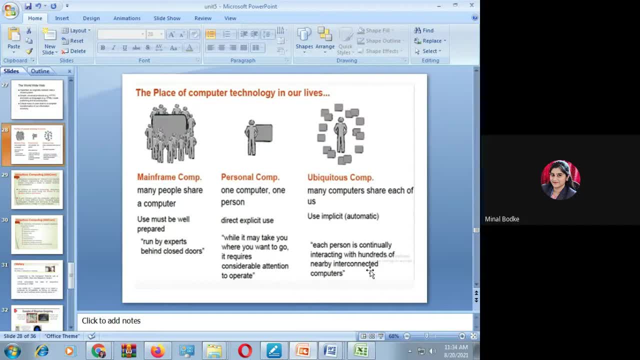 Okay. So what the sensor will do in this case? Okay, the sensor will detect the objects. Okay, in a particular room, if the light is on for a long period of time and if the sensor will not detect the objects, Okay, The sensor will not detect any object for a longer period of time. 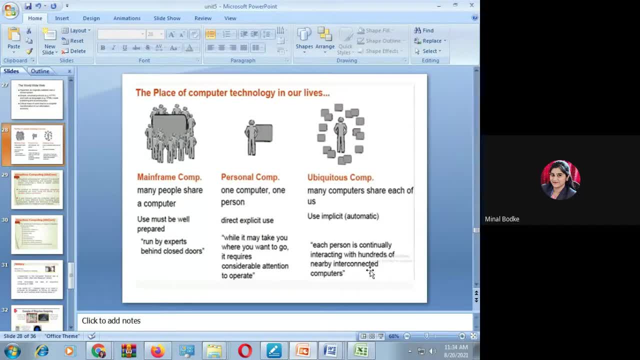 What the sensor will do. it will automatically switch off the light, Okay, and if the person is moving from one room to another room and the light is off? So in that case, if you will detect any person entering into the room, Okay, it will give the information to the sensor and sensor will process and it will switch on your light. 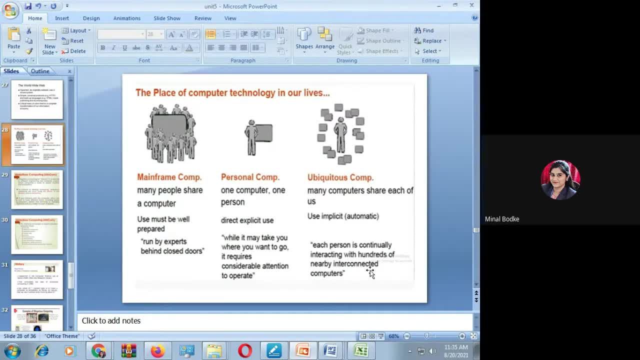 So this is nothing but the concept of what your smart home. again, in the smart home, You have the concept of lock and lock, Yes, So n number of devices which are interacting with in your day-to-day life. You can automate, automated Okay, and you can give the control to the computers. 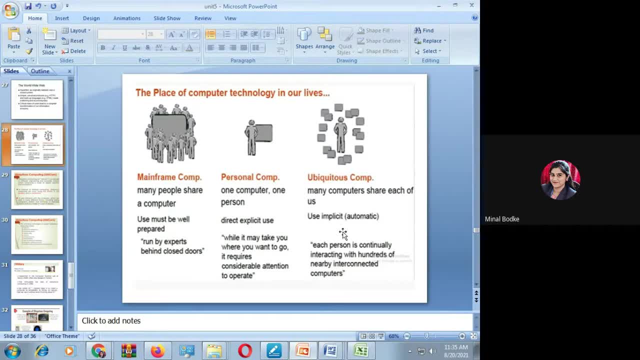 It is nothing but your ubiquitous computing. Yes, So ubiquitous computing is nothing, It is not just a computer. Okay, So, along with the computer, Okay, you are going to embed your computer technology into what your hardware system, electronic devices, or your mechanical devices. 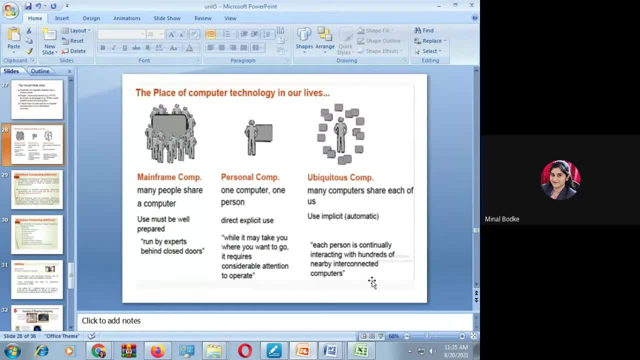 Okay, So you are embedding the software or the computer technology into a particular hardware. You can make that system as what your smart system, and you can make them to operate. Yes, So that is a concept you have in what your ubiquitous computing. So now let us see the definition. 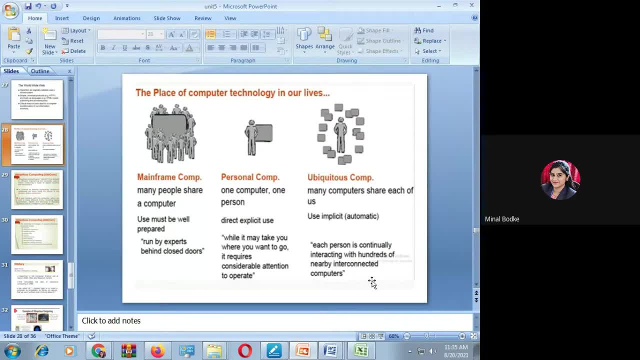 So can you tell me some examples? Yes, you are using in your day-to-day life Seeing ubiquitous computing every time. you cannot see computers everywhere. Okay, So it is embedded in something like software or your devices? Yes, So see here. 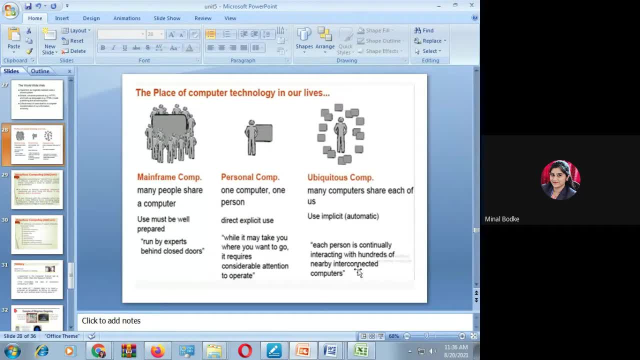 What is the definition? Each person is continuously interacting with hundred of nearby interconnected computers. Yes, So see the size of computer as compared to your personal computer, mainframe computer and n number of generation. The size of the computer is also reduced, So it is available everywhere now. 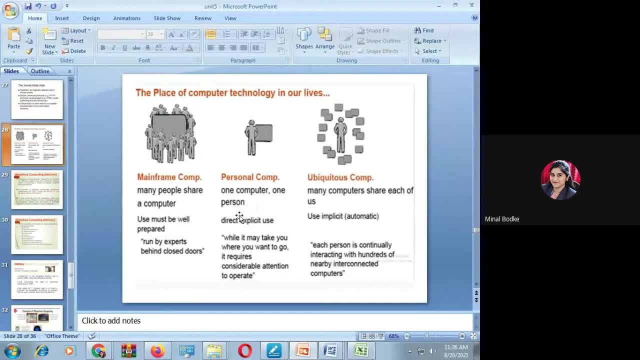 So, instead of the personal computer, what was the scenario? You have to sit in the front of the desktop or PCs or laptop You have to carry if you need to do some computerized work, But in the case of ubiquitous computing, you can be present anywhere, anytime, and you can perform your tasks. 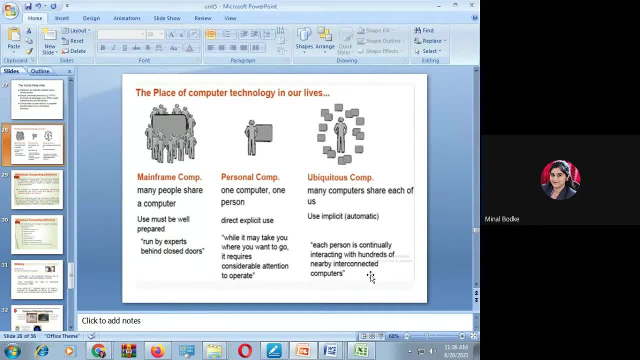 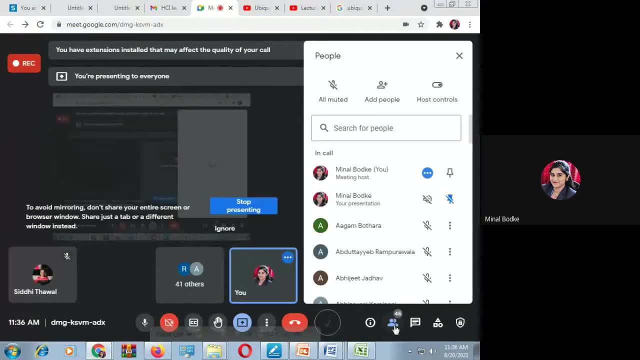 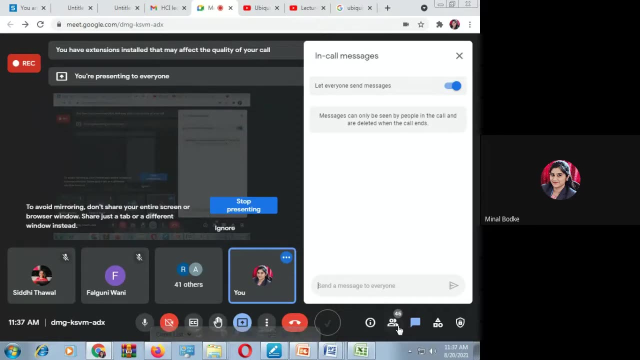 Yes, So can you tell me some real-time examples? Yes, Abdul. Yes, ma'am, Can you tell the example, Real-time example, of ubiquitous computing, Ma'am, are sensors? Sensors, Yes, the sensor is a part of the component which has been used in the processing of your computing. 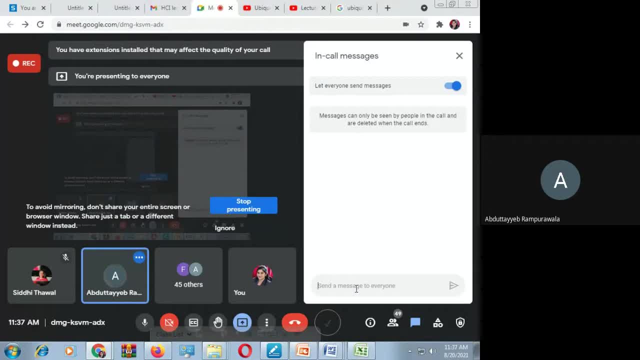 devices which we use, like, uh, wearable devices, watches and on. yes, right, so your apple watch? yes, i think. so everyone is familiar with that apple watch, okay, that alerts your user to receive a call, or when you have a phone call and you can receive the call. okay, so this is also the example. 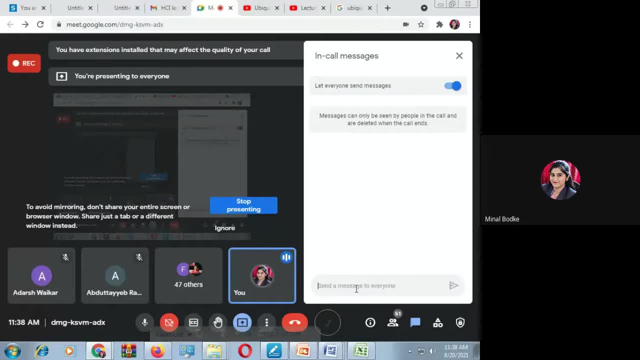 of computing, ubiquitous computing, again. your smartphones like amazon eco is there, google assistant is there. it is also in a real-time example. again, you have self-driving cars, then smart locks. then again, can you tell me such type of examples, ma'am? can we consider our railway station lightning system in that? 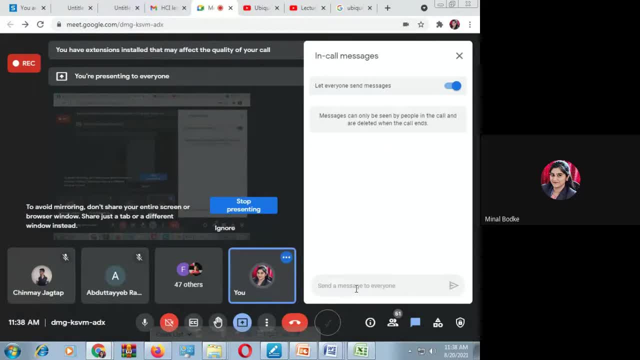 yes, yes again. your toll system- okay. whatever toll system you have on the highway is. that is also a part of your ubiquitous computing- than your this app like traffic lights- yes, traffic lights, right again. your this app, life 360- okay, which is used for tracking the location. 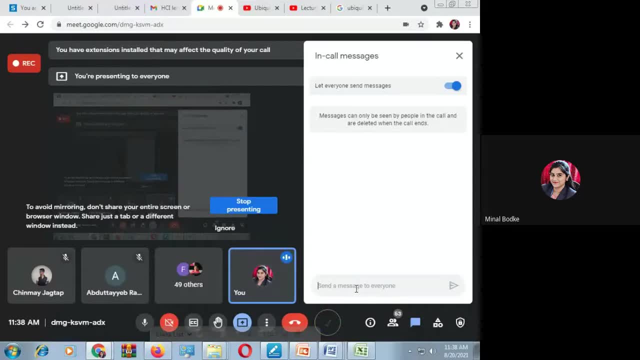 of the user, then speed of the car. yes, so there are n number of applications. you are interacting in day-to-day life. so, uh, have, do you know the concept? so in the fridge also you can have your ubiquitous computing. okay, so in the fridge also you can insert the microprocessor, or the cheap you can. 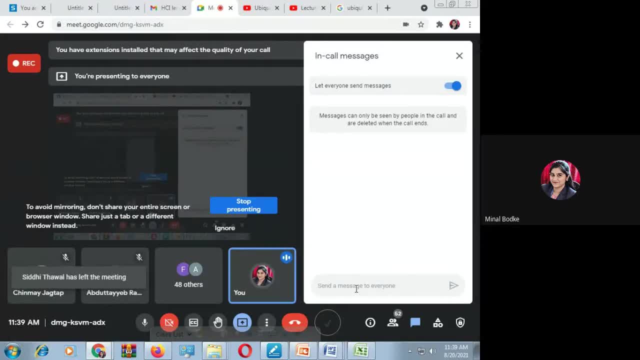 embed so what the sensor will tell here by using this computing. okay, if you embed this, the fridge can tell you the information, like if any of the food atom in the fridge gets expired, so it will give you the indication or message onto your phone that some atoms from your fridge is getting expired. 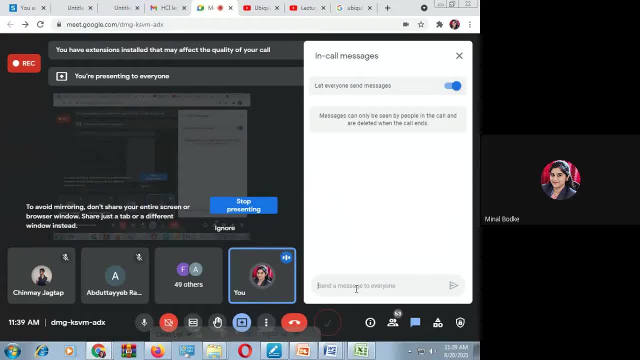 or some expiry date is near on, or it can give the informations, like it will sense the food item and it will tell the number of quantity, whatever it is present in the fridge. okay, so, using all this, what the user can do: he can buy the quantity or he can remove the expired things. 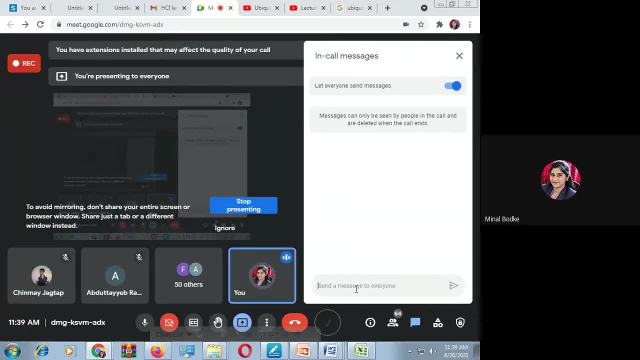 okay, so what this had made? all your human capability of recalling, memorizing, has been reduced. okay, and you are using most of the automation part here. yes, so again you can take the example of this pair of glasses where you can see 3d objects, 7d objects. your virtual reality is 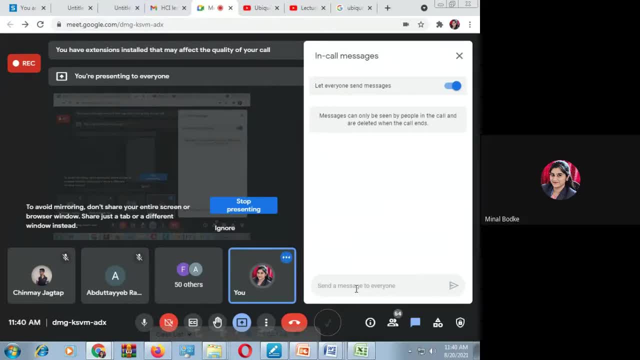 also example of what your: ubiquitous computing. yes, and now what? why it is included in hci? because the interface which you are developing, okay, for the ubiquitous computing, so it must be according to what all the users, okay, so all the devices like your fridge, your, this pair of 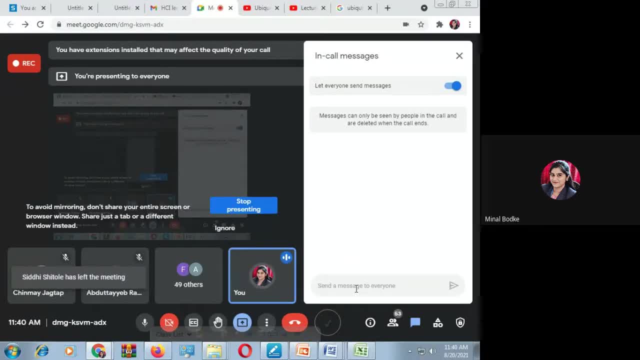 glasses, then toll system, then you are this apple watch. yes, it is user friendly to all the men, okay, whether it is all the people, whether it is computer literate or a common man, okay, so how the designing must be of this ubiquitous computing? so it must be according to your hci roots or hci. 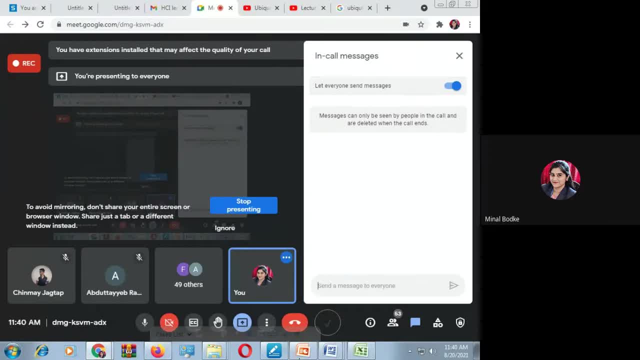 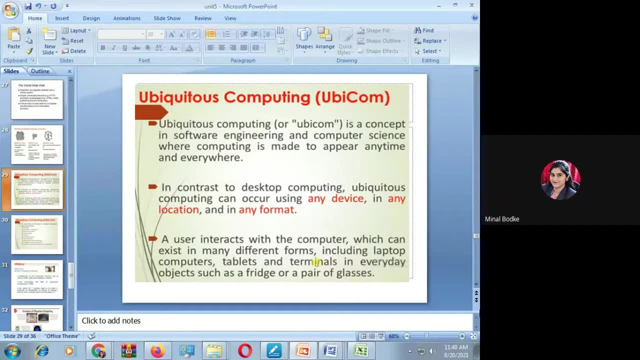 principles. okay, so next we are going to see what is the definition of this. so what is ubiquitous? it is a form. so it is a concept or a combination of what you are going to apply, the concept of software engineering and computer technology. because of that, you can provide computing. 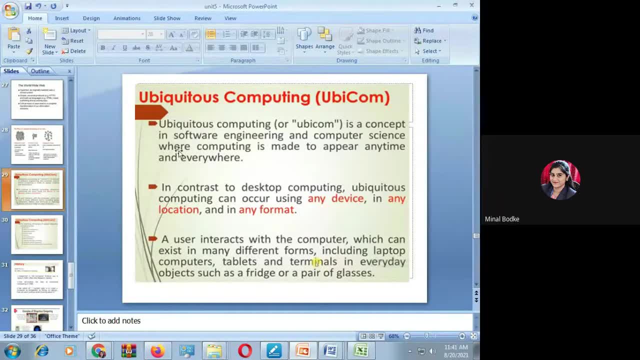 anywhere, anytime, for the people, okay. so now only the user or the people think computerized technology means what? always your desktop, okay, so instead of that, in ubiquitous computing, you can embed your technology or the computing system in any devices, in any format, in any location. okay, so just, we have discussed the example of fridge pair of glasses and total. 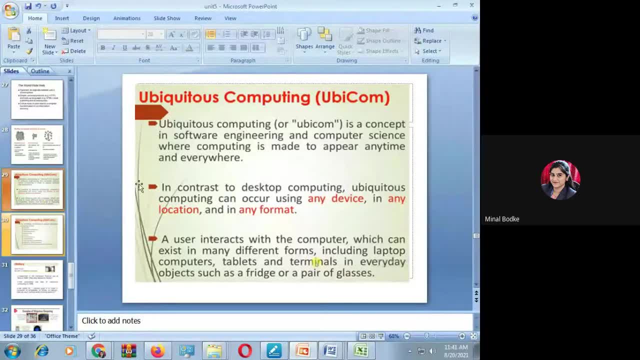 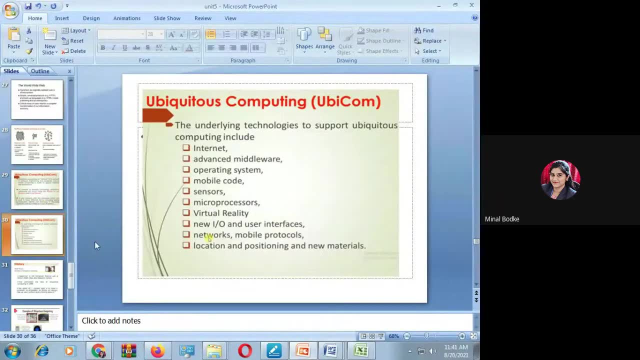 system than your mobile. yes, so this is the definition you have for what ubiquitous computing. next is what now, when you go for implementation of this computing? okay, so you just don't require the computers or your chips, but you require n number of technologies. okay, to support this. 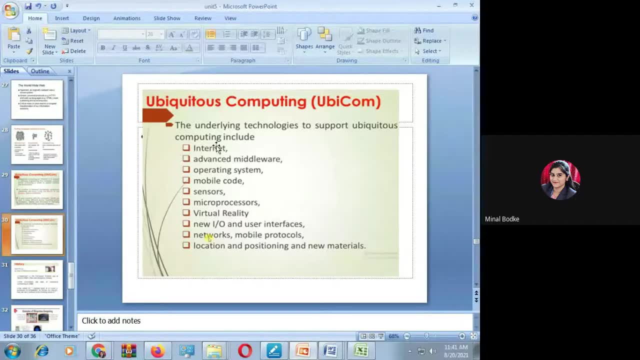 computing, okay. so what are they? first is the computer? okay, then the my computer. okay, then the your internet. you require, the first and important thing you required here is internet connectivity. okay, then middleware, okay, middleware means what it is going to provide, the interference or mediator. you can say then operating system, mobile code, okay. so mobile code means what? whatever code or 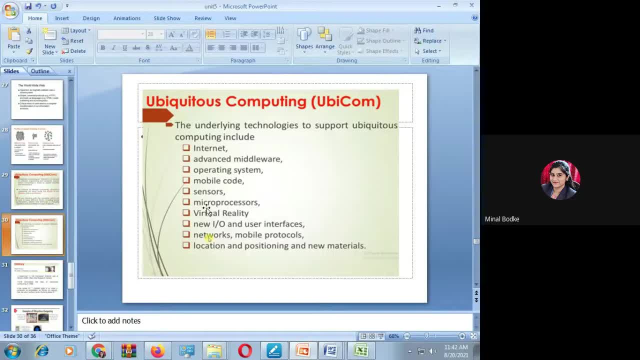 application you are going to develop to operate in this computing, it must be feasible and compatible to n number of devices. okay, and sensor is again the important part of your computing. okay, through sensor only you are going to get the input. you are going to process something. okay, and then you are going to give instruction to what your microprocessor or the chips you are. 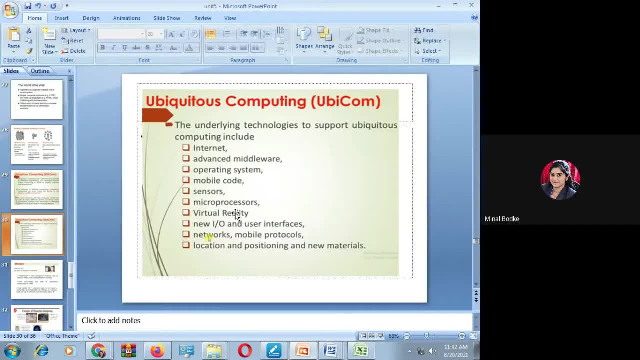 going to install. then again comes your virtual reality. then you input, output devices and proper user interface. you must have okay, networks, mobile protocols. you need to have location and positioning system. you must have see all the technology, okay, so all the computers, what you are going to get, the input, you are going to process something, okay, and then you are going. 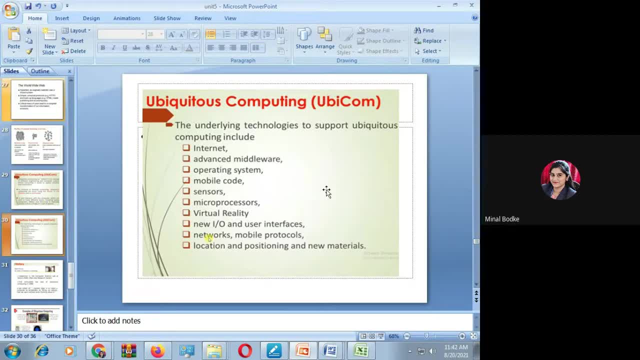 whatever we are talking about, or all the electronic smart devices are interconnected with each other through the networking concept. so when you go for this computing, you must know the basic of computer networks. what is your lan vlan? ad hoc networks, yes. so using ad hoc network, then wide. 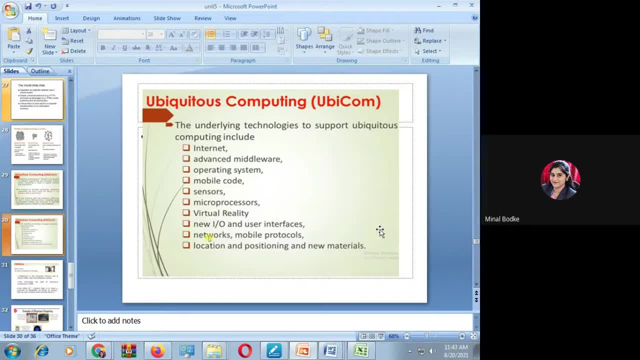 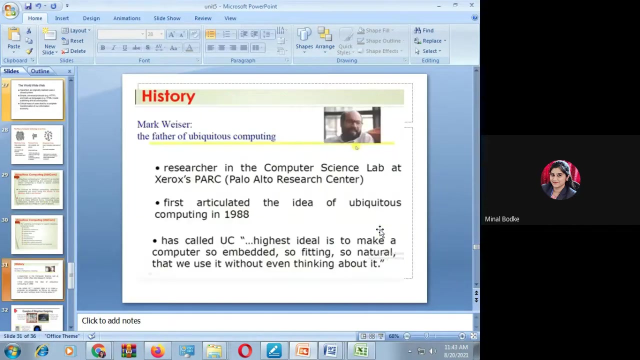 area network. you're this, typical computing is done. okay, so you can say, in all you need the knowledge of your computers programming. then again, your networking, your embedded system means it comes the concept of your electronics devices, okay, so all the ubiquitous is a combination of what n number of domains. okay, so when you embed, okay with your software, the networking part, it. 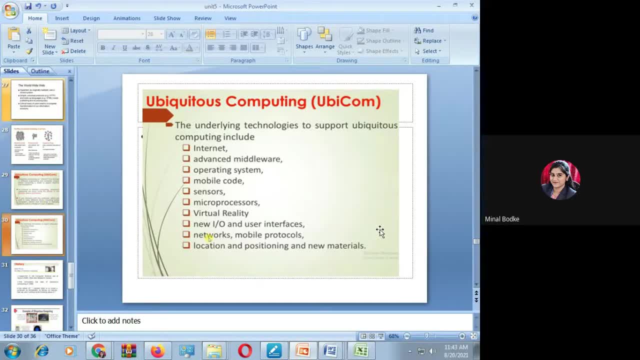 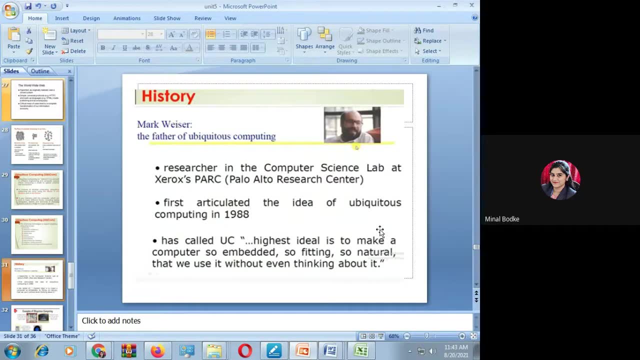 is also known as what your pervasive computing. okay, the second name you have for this concept is what pervasive computing you? okay. so who is the father of this? the mark wizard is the father of what your ubiquitous computing, and it was first developed in what? in the computer science lab? at what year? xerox park lab. okay, so it. 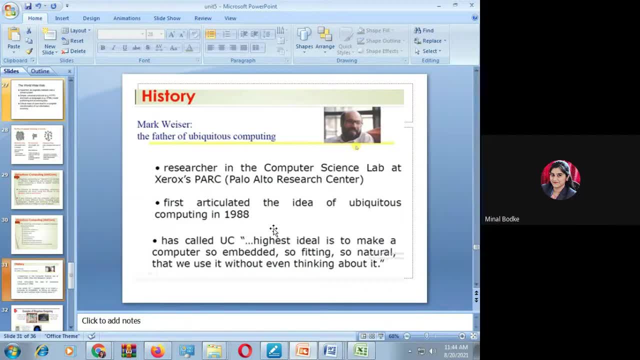 was first developed in in which year? 1988? okay, so what was the aim of the scientist? okay, to make a computer ideal in such a way that it can be fitted, okay, in any natural objects or devices. and even a normal uh user cannot understand whether it is a computer or whether it is a device which. 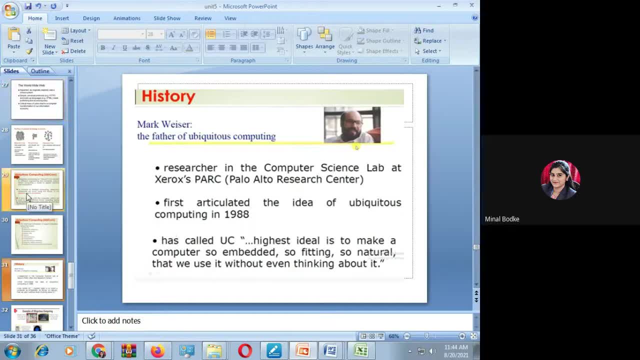 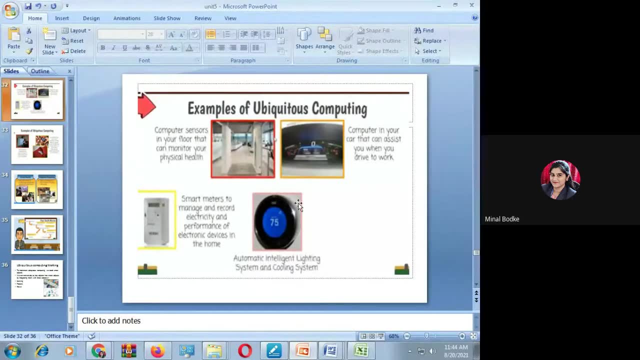 is operating it okay. so this is a history you have for what ubiquitous computing. now see, you have a number of examples like this company computing is also used in what your healthcare system, your transportation system, your defense, okay. so this is example you have where the computer sensor are. fitted on the flow with your home rằng you put it on a computer having the- thank God, this the flow, the data is so direct so that it doesn't derail cuz right now. this is a good way to at least where the system of the device, the company cariders, get to the accuracy of the hive. very well, voicing this and then you'll need a lot of things to understand rather than just seeing what human is, computing and, um, any other Oregon and it don't understand it. ok, but yeah, really simple. I think the next caseThank you have h sex in this and see why there is a. 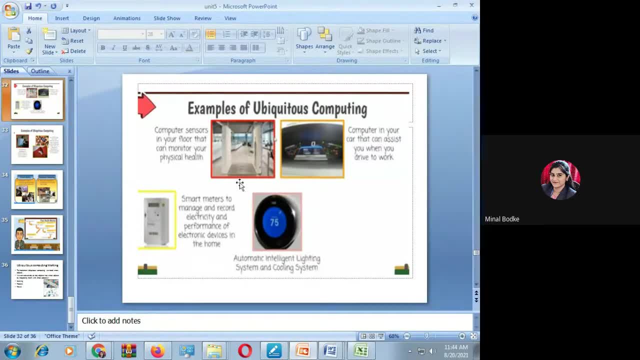 it can monitor your physical health. so when the person move in and out of this floor it will detect the temperature, then vp and all that. so using sensor, you can do this again. the computer in your car can assist to drive. okay then, automatic intelligent lightning system and. 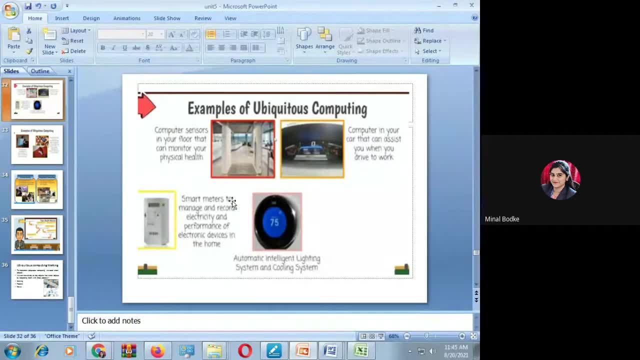 cooling system you have. okay, then smart meters to manage the electronic devices performance you have. so a number of example you'll get related to what your ubiquitous computing. okay, i'm going to show you one video. you have to observe that what is the latest trend in this? you will see in that video. 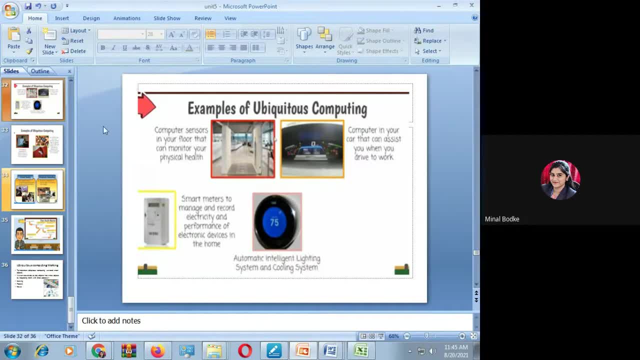 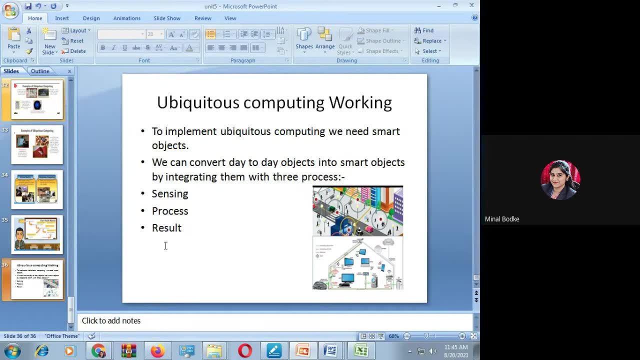 so two to three example is shown. okay, just before going to that video, i want to tell you the process. so what is the process of ubiquitous computing? okay, now to implement. so when you enter in a particular room, can you tell the fan or the bulbs we have in the room as a smart object? 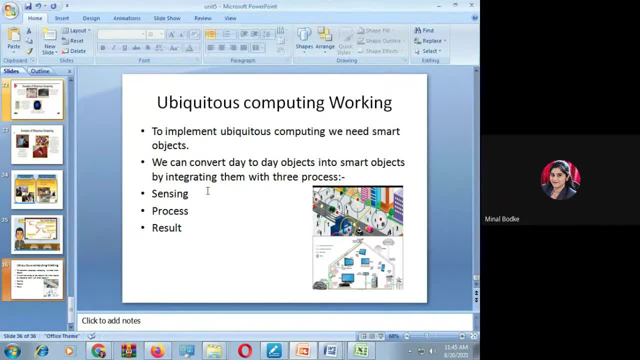 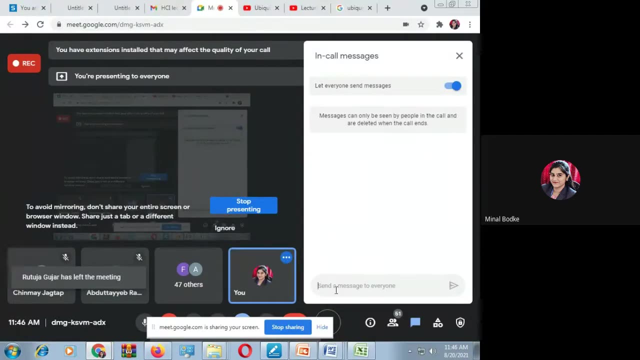 yes, whatever tube lights or the ac you have, okay, it is a smart object. yes, whatever fan lights you have in the home, do do it get automatically started or you need to switch on and off? we need to shoot it. yes, we need to do it to see this. all whatever things we have, okay it. 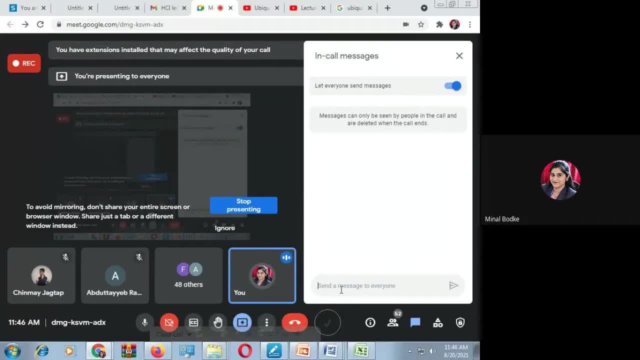 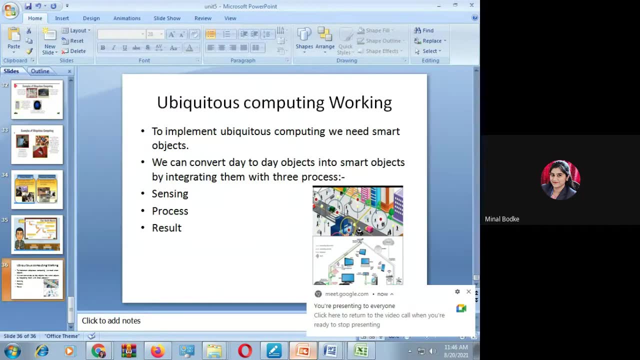 is ordinary object in the environment, whatever we are operating. okay, so you need to convert. for ubiquitous computing, you need to convert this ordinary objects into what are smart objects- okay, so that it can operate automatically. so, whatever your fans, tube lights, ac fridge, whatever examples you have in day-to-day life, you need to convert first into the smart object. 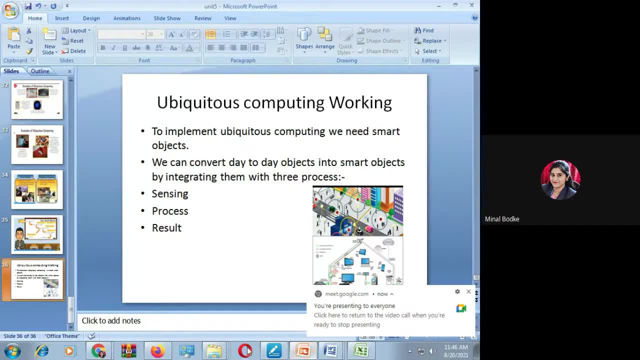 okay, then only you can perform what all the processing or computing. okay. so to convert this, what you need to do, you need to perform this: three steps. okay, you need to integrate with them what a microprocessor or the chips? okay, and you need to perform this three operations. that is, sensing, process and result. okay, 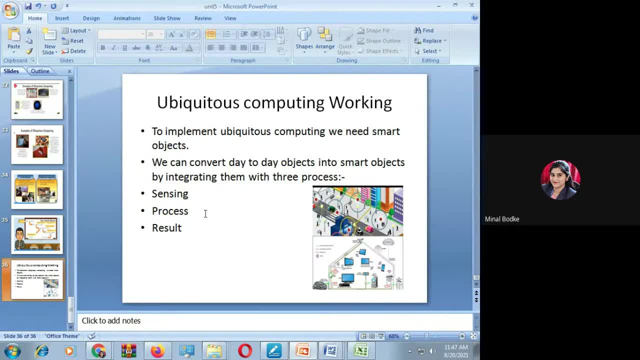 and again. one more important part here you have is actuator. okay, so actuator is something which is going to perform some actions. okay, when it sends something, it will analyze, process the information and result will be displayed to you. okay, through the actuator. okay, so sensor, what is here? the sensor will sense the object. 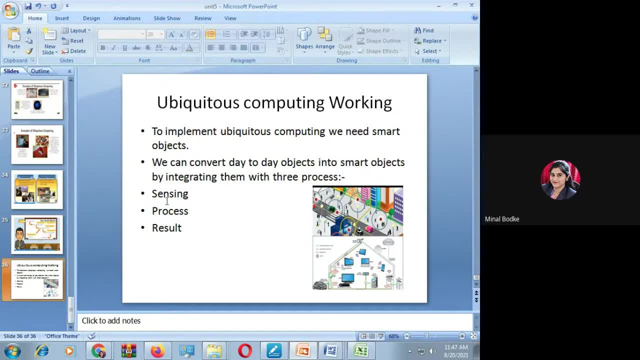 from the environment and the sensor is going to have analysis. okay, and for analysis purpose you are going to use your machine learning here. okay, to analyze. you are going to a certain set of classification. when you receive the object, it will sense which type of object it is and it has some threshold values. okay, and depending that, threshold values. 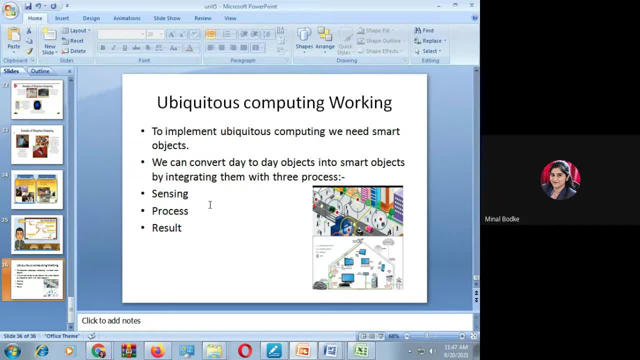 you are going to compare your object and then you are going to process and then you are going to produce the result. okay, the result can be in the electronic form. it can be in the form of your software's or the instructions or the actual actuator who is going to perform some actions. okay, so let us see one video. okay, 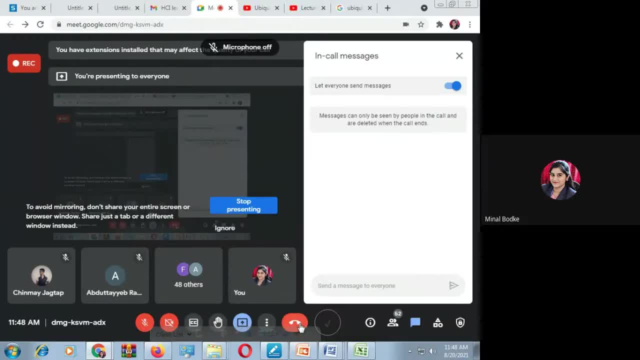 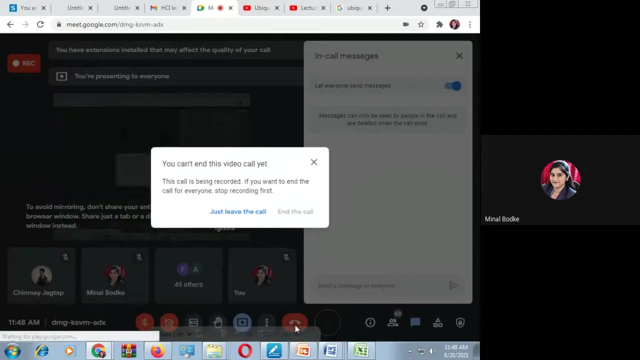 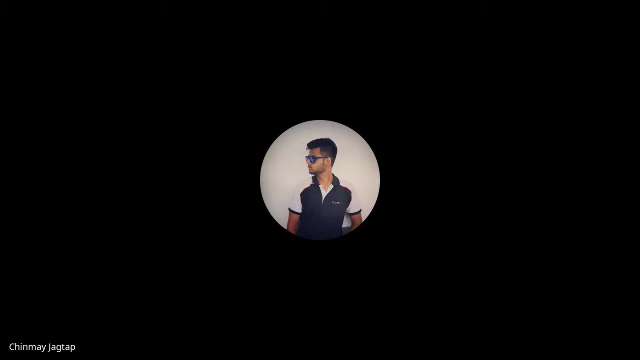 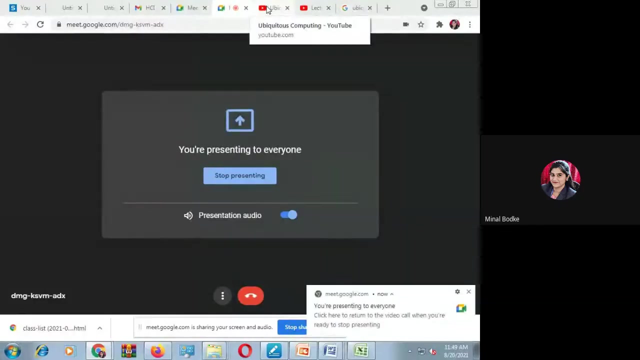 so let us see one video. you, Ah, see. this video will tell you what is the current train going in the you become computing okay. so what? it will be okay in the coming days. so, just having present the video, you, you, you, is the screen visible? is the screen visible? 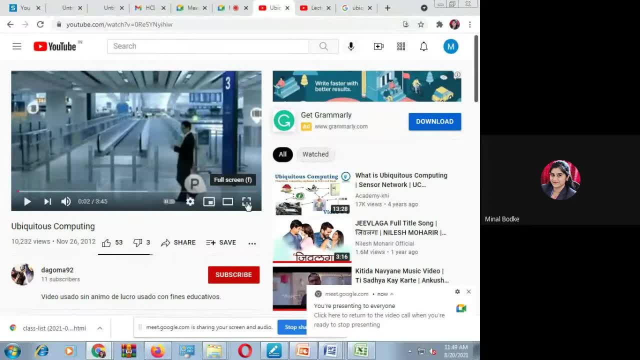 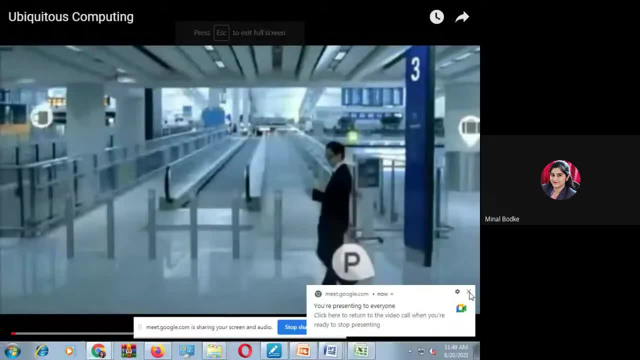 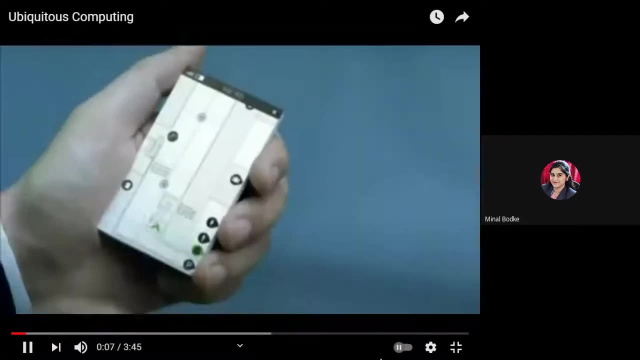 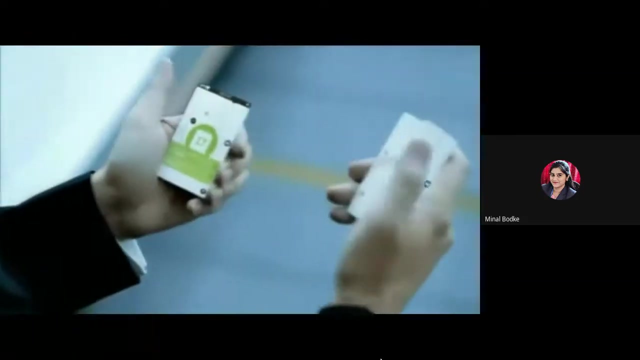 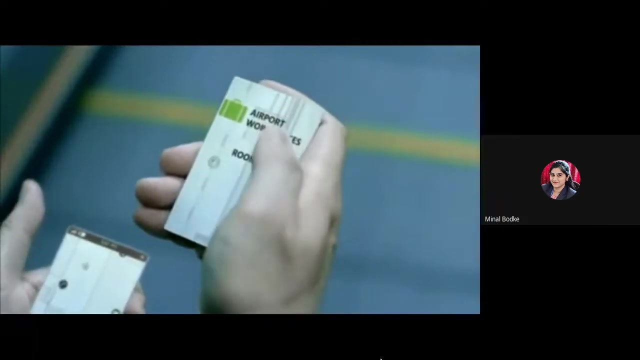 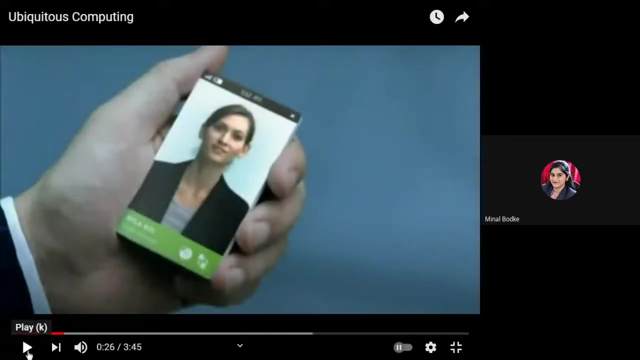 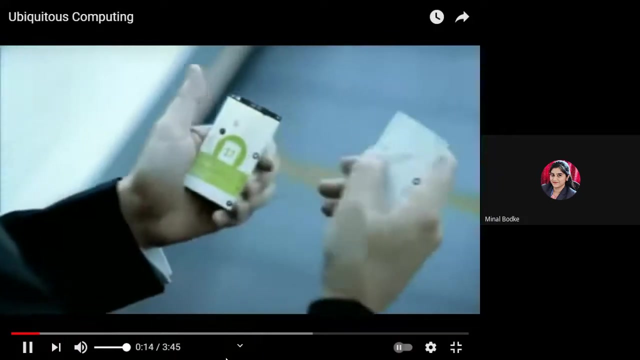 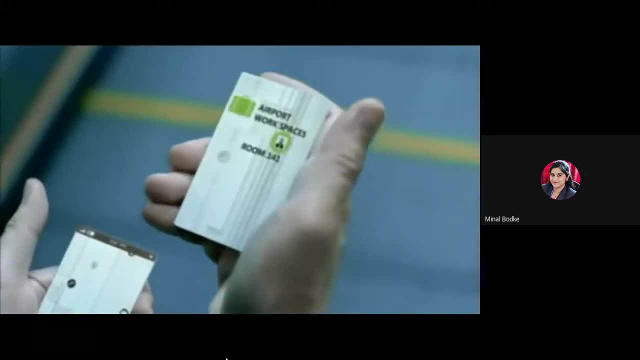 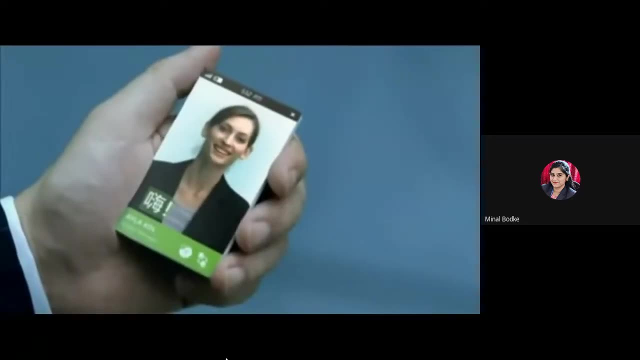 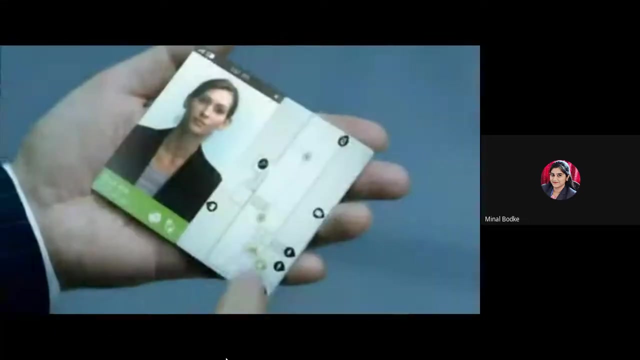 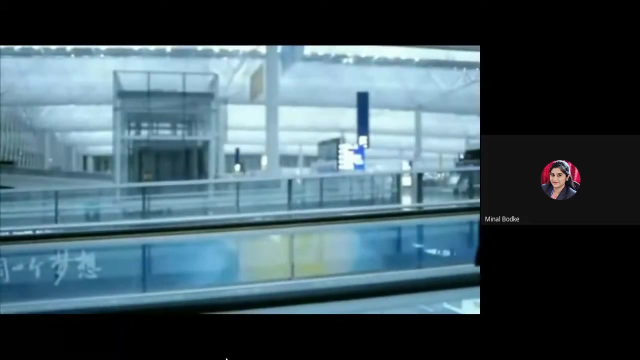 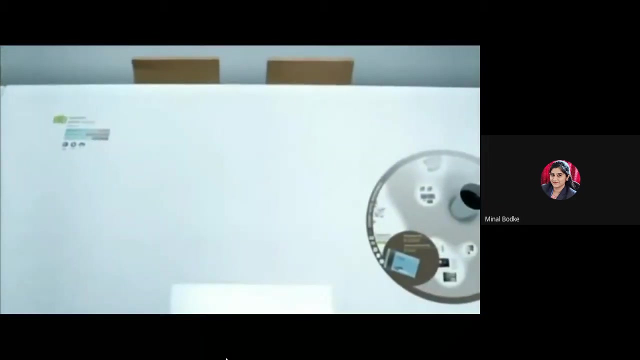 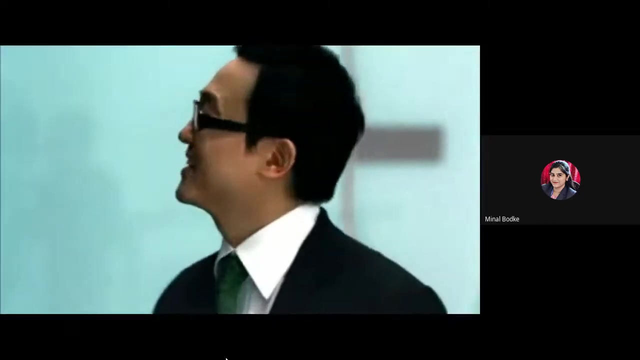 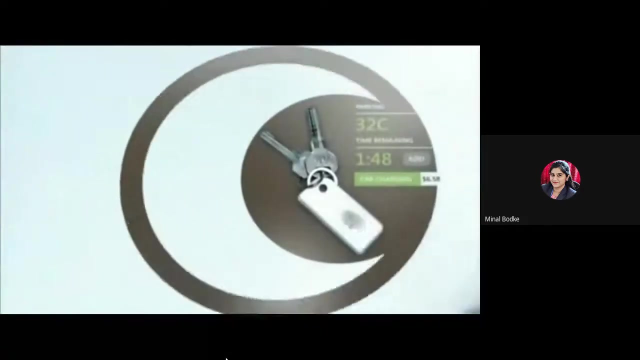 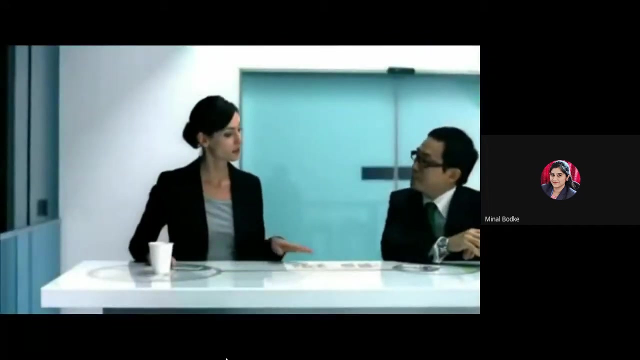 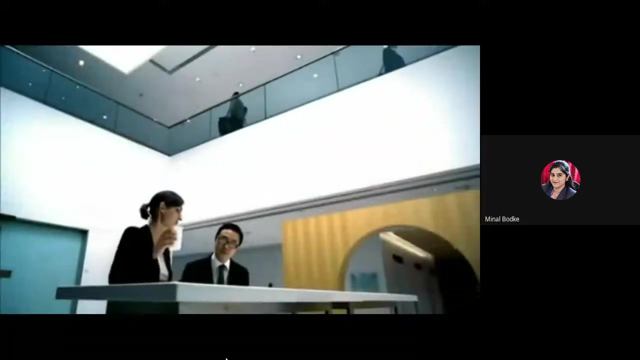 today. I know what my listeners have been understanding: just watch the video carefully, see. observe the video carefully, because you have to tell me your observation. okay, because you have to tell me your observations. okay, see if you want to watch the review. Thank you, Thank you. 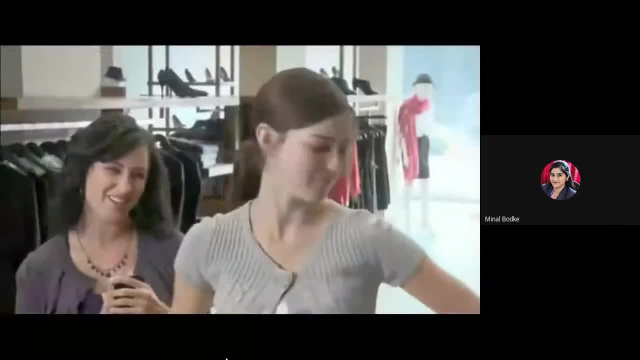 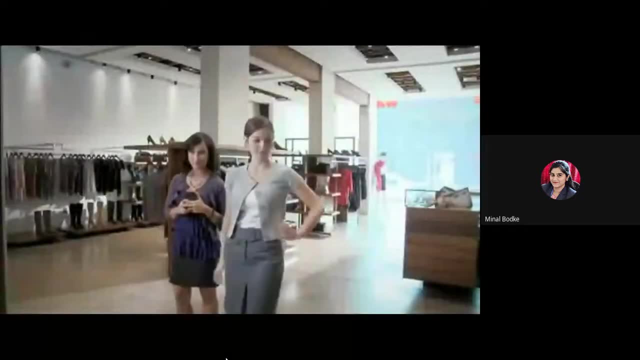 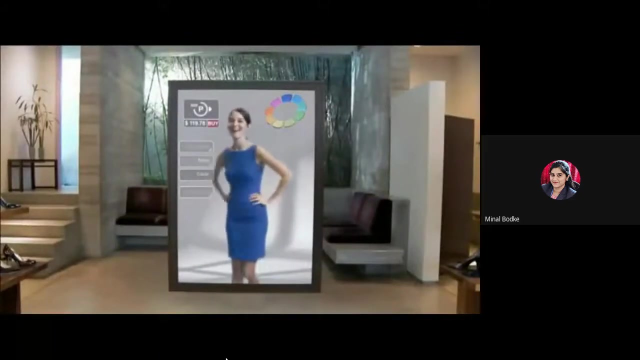 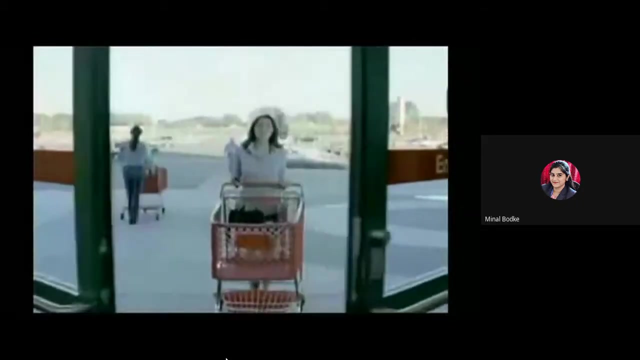 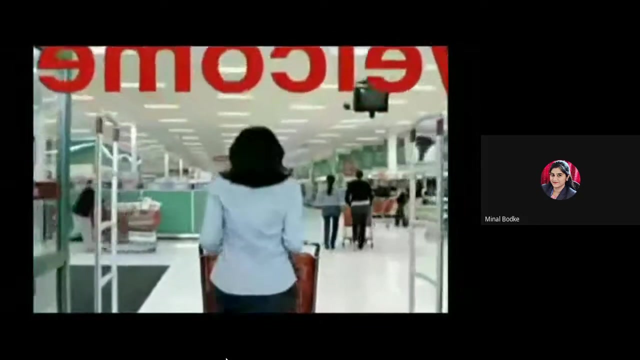 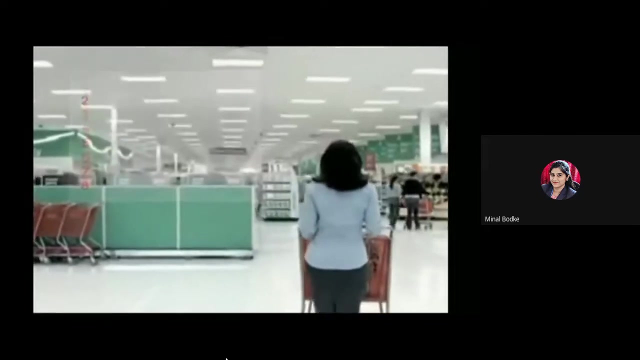 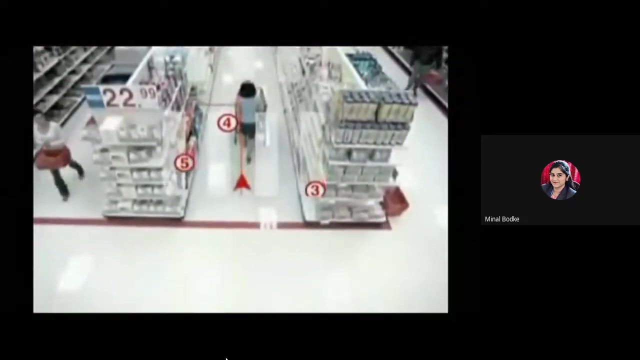 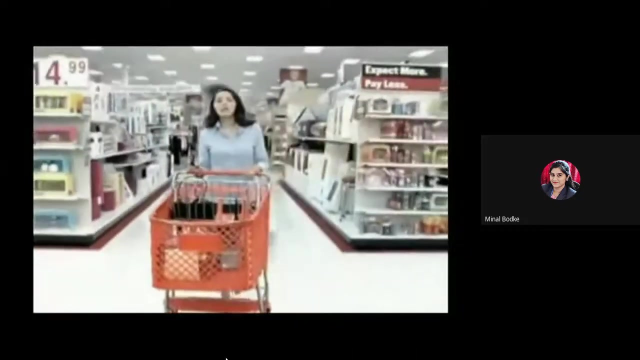 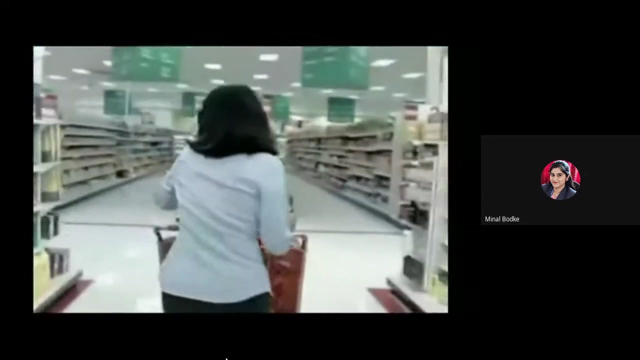 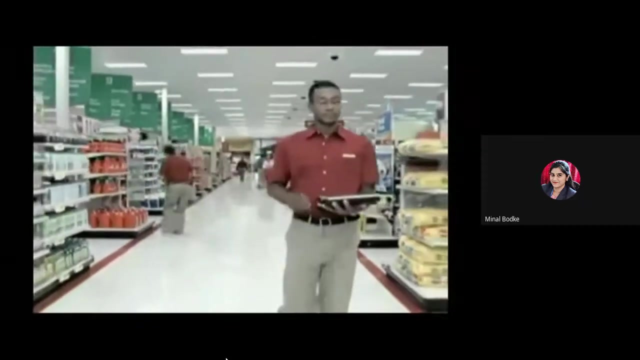 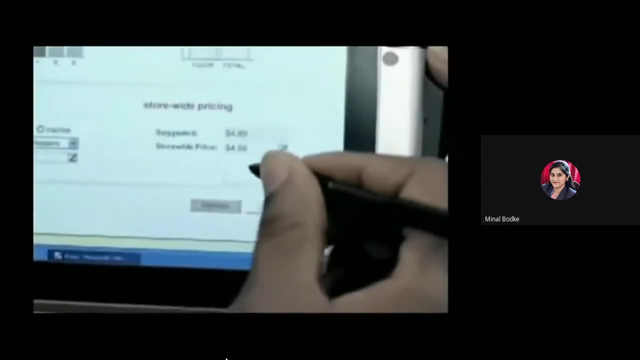 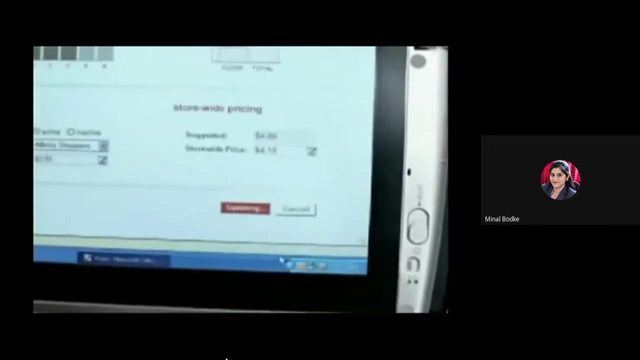 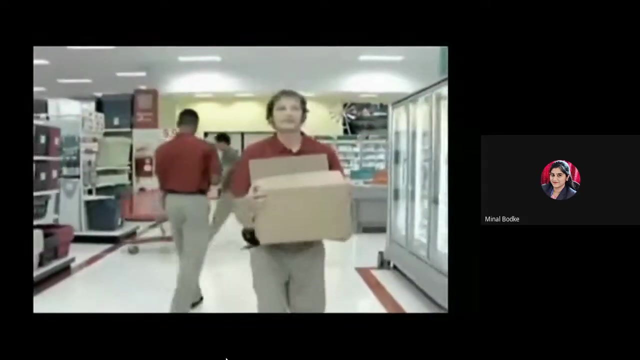 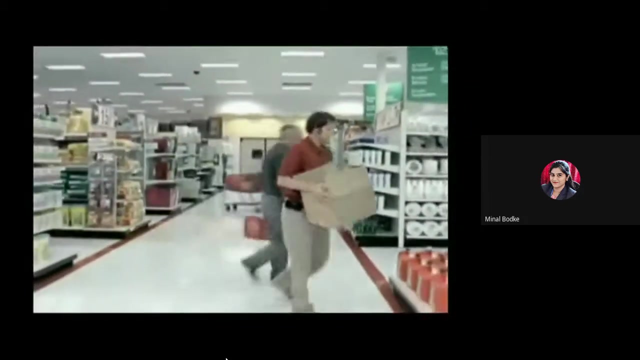 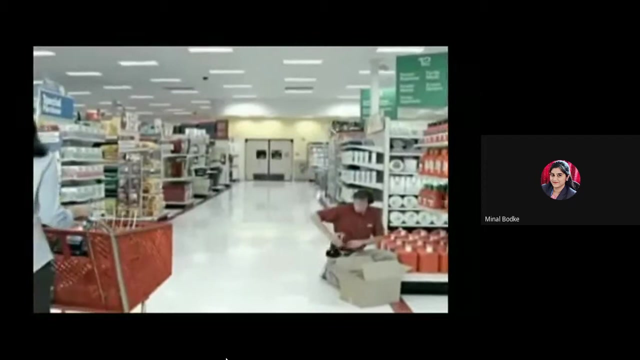 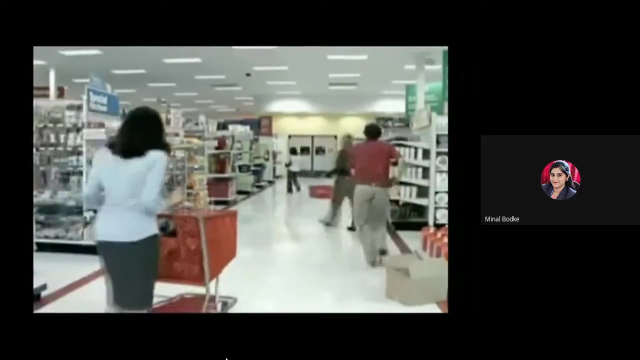 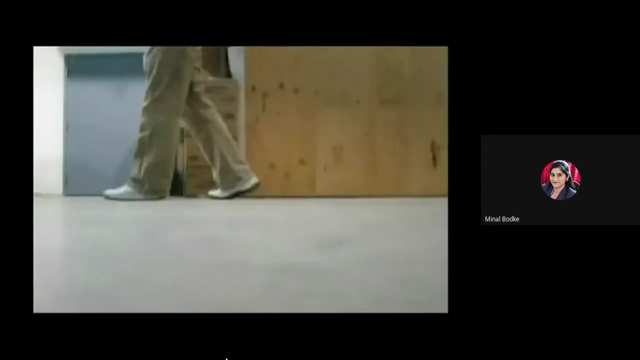 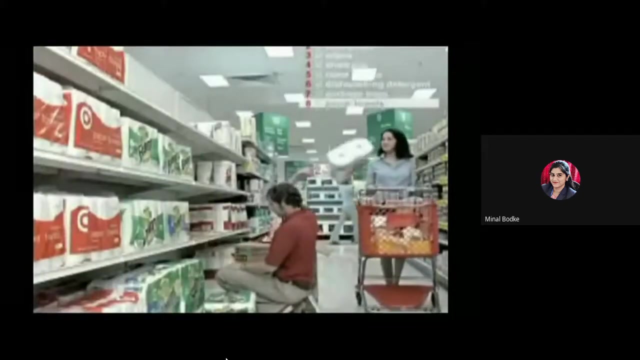 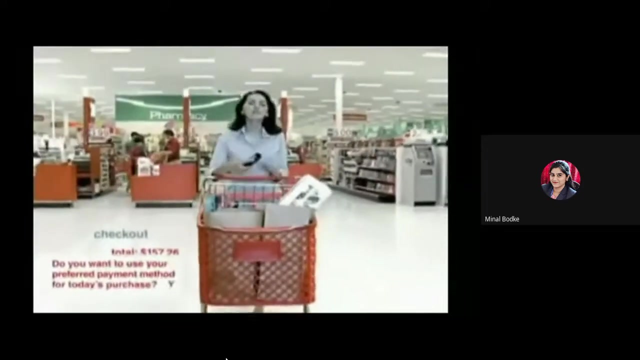 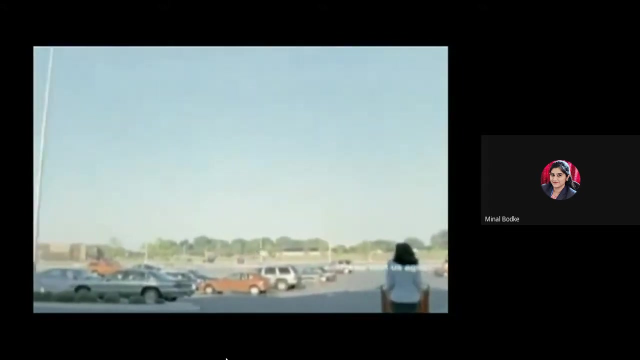 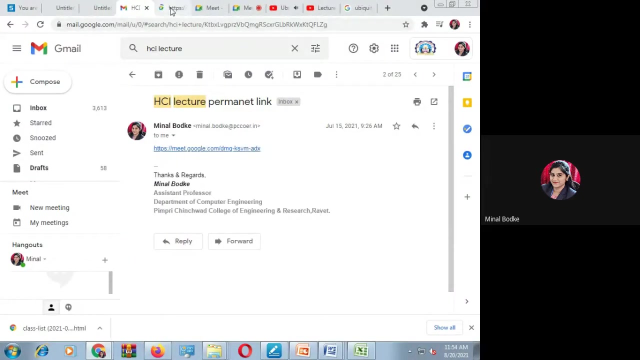 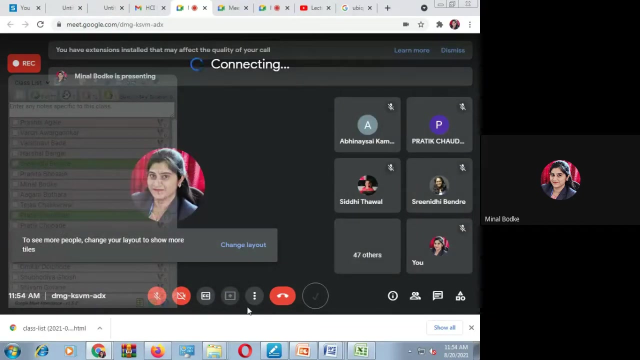 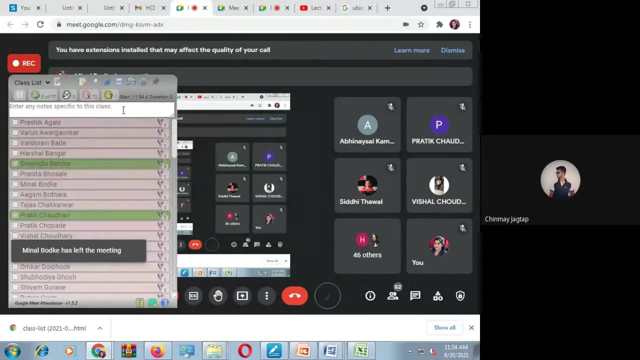 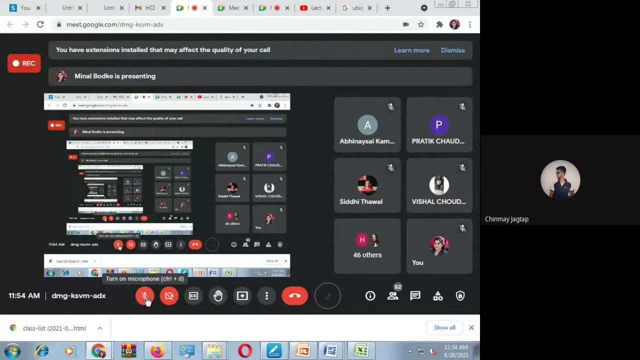 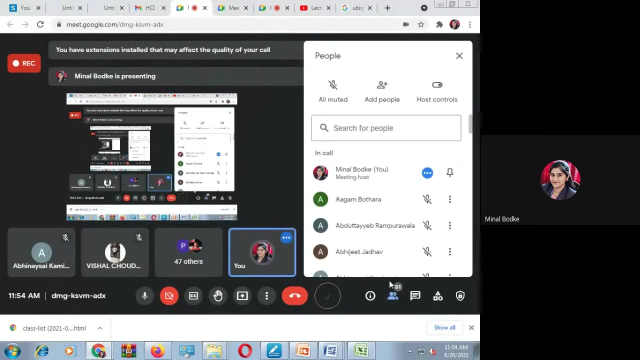 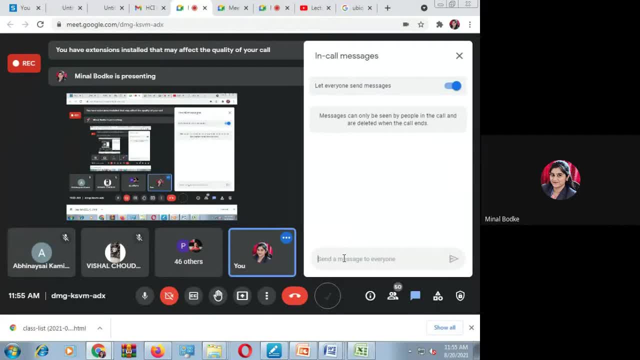 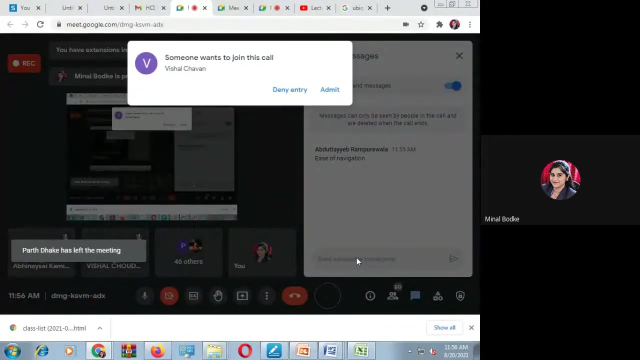 Yes, Can you tell me? Can you tell me, Mansi, are you there? Yes, Ease of navigation, But can you tell me your observation, Abdul? Yes, Yes, anyone. Yes, Wave, is there a wave? See, don't leave the meeting. 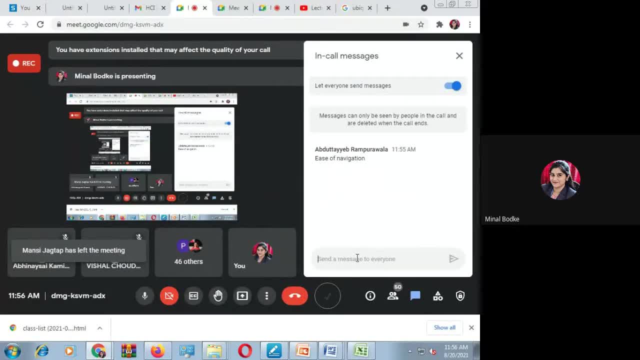 if I'm asking the question. Yes, Yes, Mansi, Yes, Can you tell me your observations? see, in the first case, when the person- okay, the person was there who arrived at the airport, okay, so what information he's got on the phone that he has got the information that? 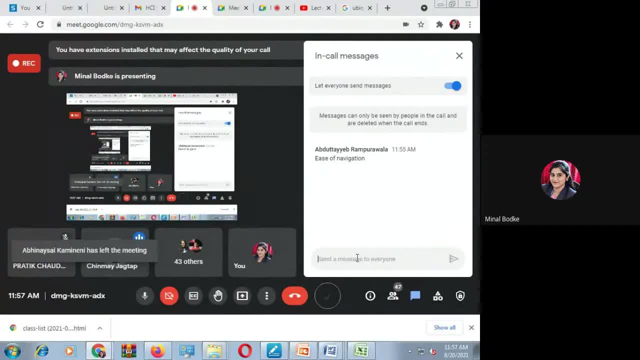 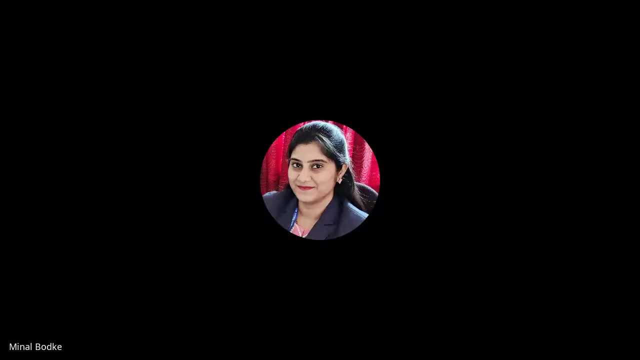 okay, now my voice is clear. okay. so what is the observation? in the first case, when the person enters the airport, okay, on his cell phone he has got the information that whom he should meet. okay, so, after getting the information where the whom he should meet, again he has got the information that where that person is. 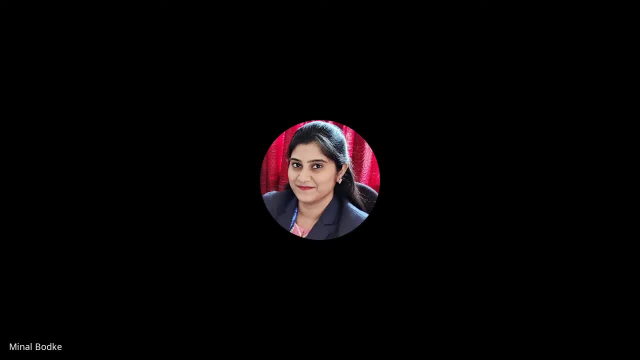 located. so again, the navigation was there. so what is the result of this? okay, much of the time is saved here, and you will get what easily information instead of searching where that person is setting, then again locating his position. okay, so this task was easier. okay, with the computing. next is what you have seen. the next: 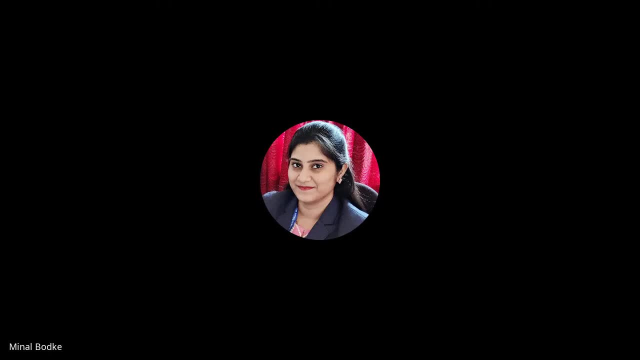 was what two girls were shopping. okay. so instead of going to trial room and trying for different types of clothes and coloring, you have just okay with the use of ubiquitous computing you have through the interface. you have just tried the different types of clothes again in the third. what was that? can you tell me the observation? now for the third. 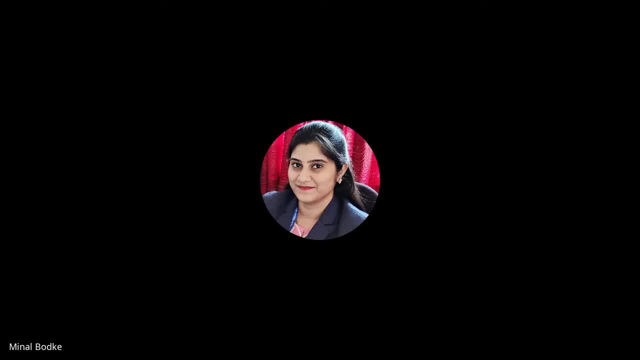 case, yes. third case: can you tell me? yes, Shreeni D. Yes, Rutuja, Yes Rutuja, Yes Rutuja. yes, prasanna, yes, prasanna. what is your observation from the third example that when you have set up your? what is your observation from the third example that when you have set up your? 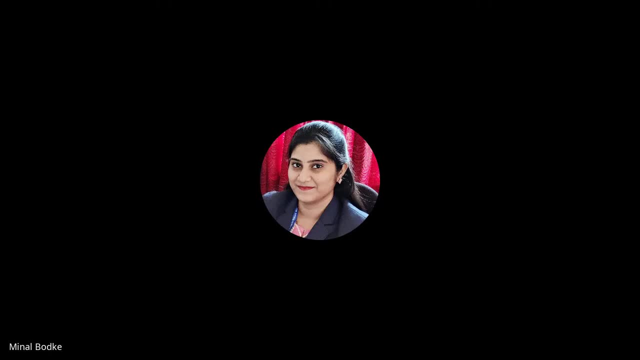 when a lady enter into a shopping mall or any this supermarket. when the lady enters she will get the information about what all the product item and also, along with that information, she is going to get the location where it is located again onto your cell phone. you will have the 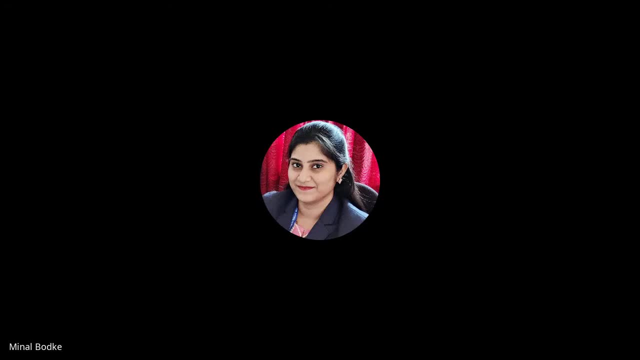 structure of all the lanes, whatever you have in that supermarket where it is located. number, then discount automatically. you will get on your cell phone: okay again, if the product is out of the stock, the supplier manager will get that information so he will again increase the number of quantity again. you have seen when she was exiting the payment so there was no need to stand. 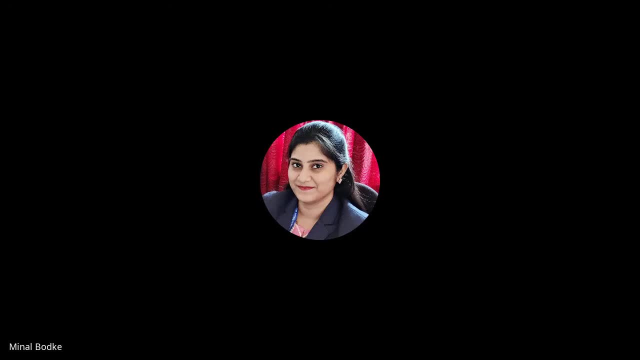 in the billing line or billing counter, the payment was done, the bill was given into the cell phone, whatever was the bill, and the billing was done automatically. okay, so there is no need to standing the billing line or in the queue. okay, so these are some of the upcoming trades or trains or the 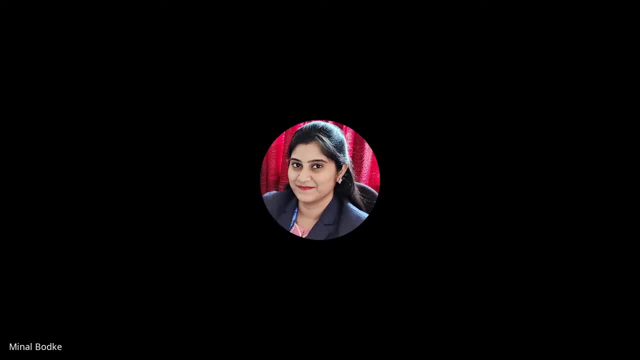 projects in what you are okay. so these are some of the upcoming trades or trains or the projects in what you are- ubiquitous computing- okay. so one more video i have of what uh, nptl, uh iit professor is there so good video. he has explained with the proper real-time example. 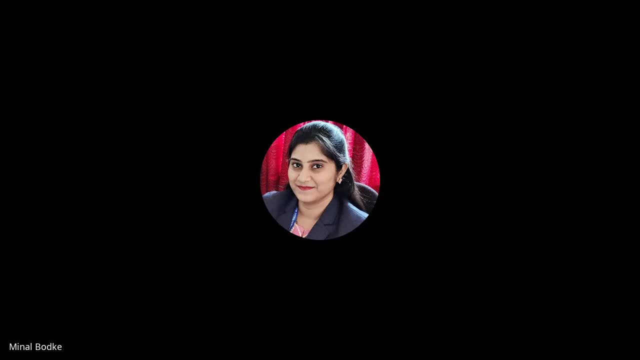 in the next lecture we will have that video, okay, so give me your attendance. yes, everyone understood the concept of ubiquitous computing up british Configuration retrofit. take me back to my and, uh, Okay, give me your attendance. Roll number one one is there, two, three, four, five, six, seven, eight, nine, 10,, 11,. 12,, 13,, 14,, 15,, 16,, 17,, 18,, 19,, 20,, 21,, 22,, 23,, 24,, 25,, 26,, 27,, 28,, 29,, 30,, 31,, 32,. 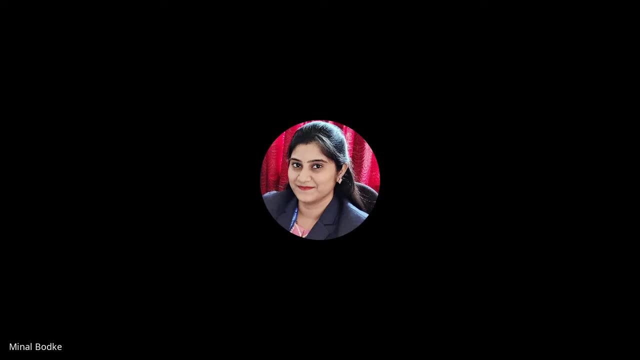 19, 18,- 18 is not there, ma'am yes. 19, present ma'am 20,. 21, 22, present ma'am 23,. 24, present ma'am 25, present ma'am 26,. 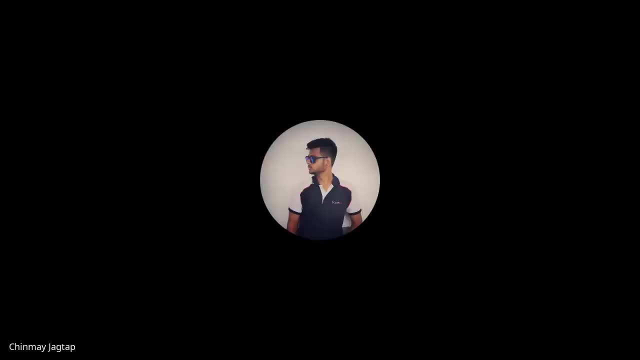 27, present ma'am 28, present ma'am 29, present ma'am 30, present ma'am 31, present ma'am 32, present ma'am 33, present ma'am 34,. 35, present ma'am 36,. 37, present ma'am. 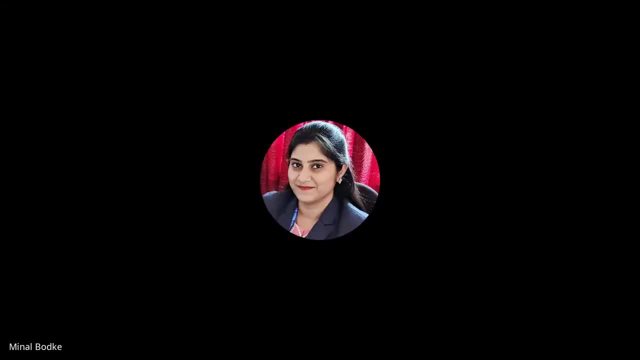 38, present ma'am 39,, 40,, 41, 1, present ma'am 42, present ma'am 43, present ma'am 44,, 45,, 46, present ma'am 47,, 48, present ma'am 49,, 50.. 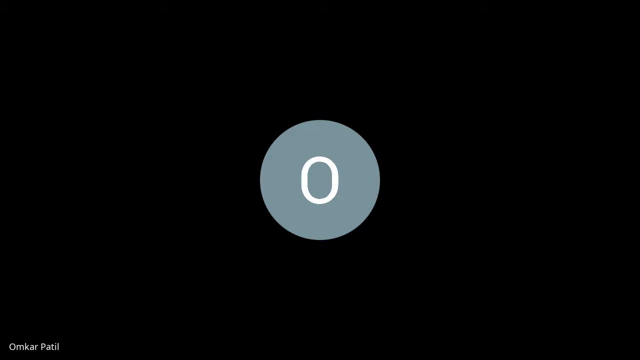 51 present ma'am: 52, 53, 54, 55, 56, 57, 58, 59, 60, 61, 62, 63, 63, 63, 64, 64, 65, 65, Yes, fast 65, 66, 67, 68. 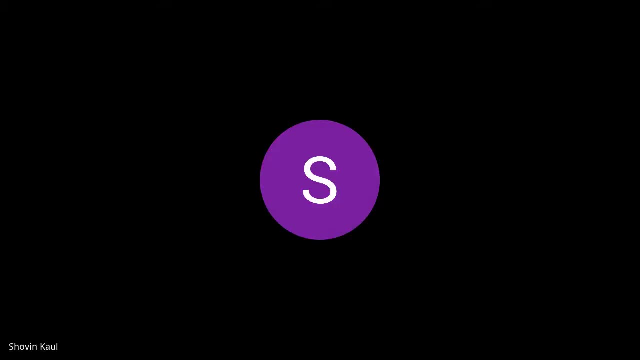 69, 70, 71, 72, 73, 74, 75, 76, 77, 78, 79, 80, 81 present ma'am. hello, ma'am. yes, yes, ma'am, I am. we have done with our PPR and digital prototype and our group is remaining.